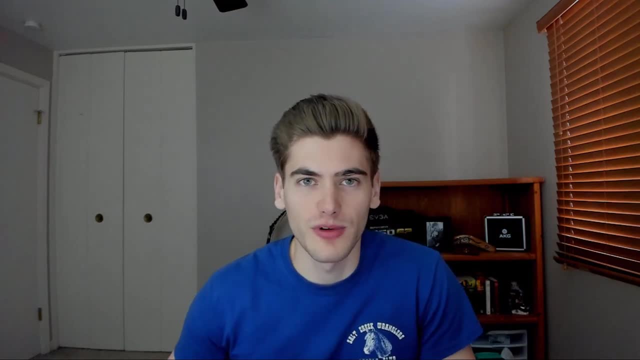 matter. These patterns can be applicable to almost any form of application. It also mentions that they're reusable, which means that you can use them throughout your application, many different times, in many different scenarios, and use the same pattern, which is really useful, because then you only need to learn the pattern once in order to reuse it many different. 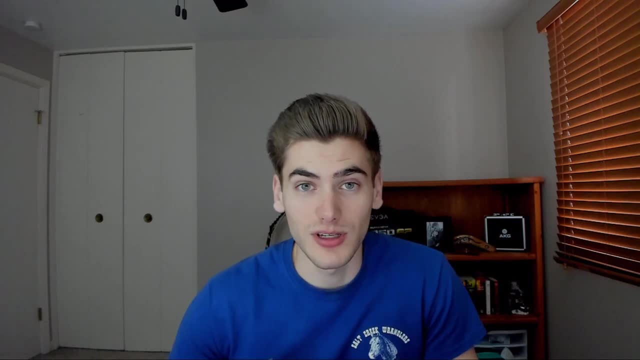 places across your applications. And then it also says that this is really a formalization of different best practices, which I think is the best way to explain design patterns, because they're really just a formal written way in order to do something that is a normal. 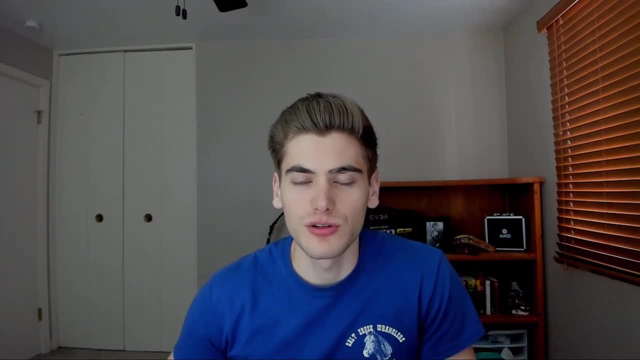 process inside of software design. So there's many different patterns to do many different things, and it's taken brilliant minds from tons of different people that have come together and said this is the best way that we have in order to do this problem in the cleanest way possible. 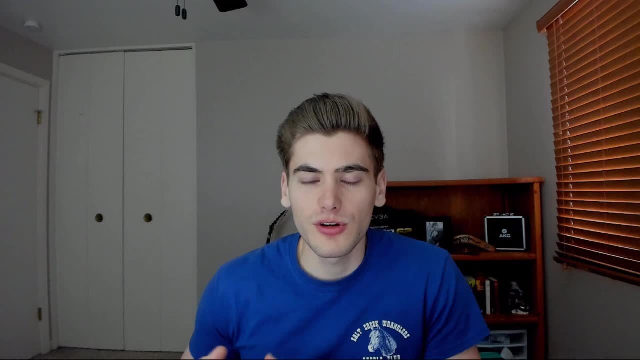 And that's really what design patterns are for. They're for making your code cleaner to use, read and less buggy and less error prone than if you weren't using these design patterns to begin with. And luckily, learning design patterns is a fairly straightforward and easy thing to do. 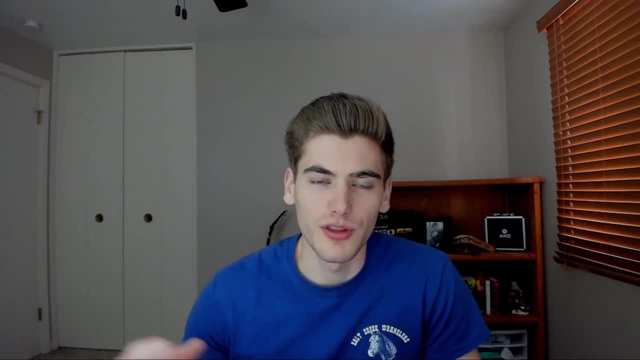 The actual process of learning the design patterns is much easier than learning when you should use them and where you should use them. I know the biggest problem that most people have when using design patterns is that they learn about them and they're like: wow, this is amazing. 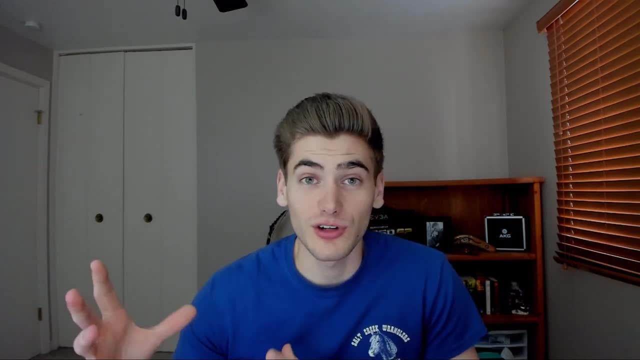 I want to use this all over the place. This will make my code so much cleaner. And they start throwing design patterns into areas where they don't really need to be, or they don't really fit, or where it may be overkill and we're not using it would be better. I know when I first learned. 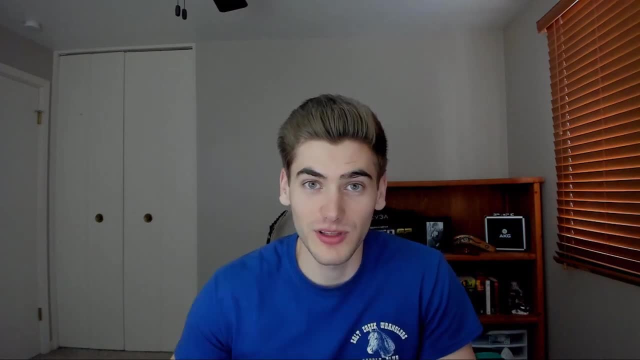 about design patterns. that was exactly what I did. I was like: wow, these are really amazing. They make my code so much cleaner, so much easier to write. I'm going to throw them everywhere, And that's what I did. Everything I wrote for a while after that was just using design patterns. 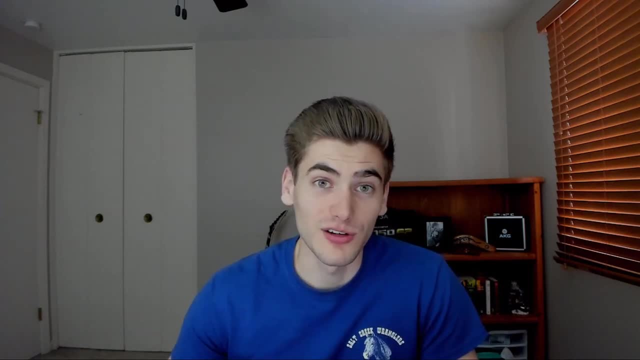 all over the place where I didn't really need them, And I made my code messier than if I hadn't used these design patterns in the first place. And this is kind of a problem, because that's really what the design patterns are there to solve is to make your code less messy and cleaner, So learning. 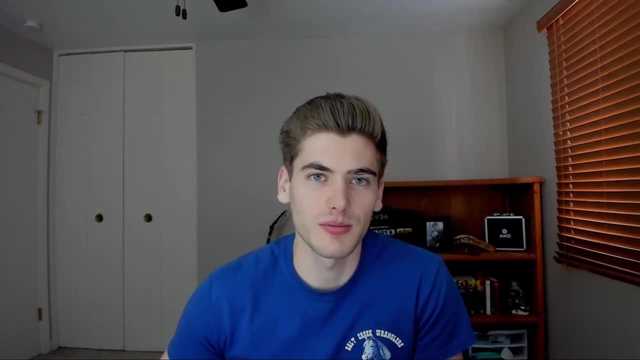 when to use them is really the hard thing when it comes to learning design patterns. This problem is that you end up using design patterns where they're not meant to be used, or overly using design patterns where they shouldn't be is some of the reason that design patterns kind of get a bad